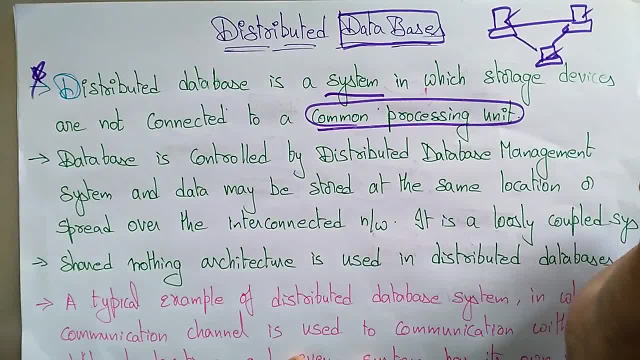 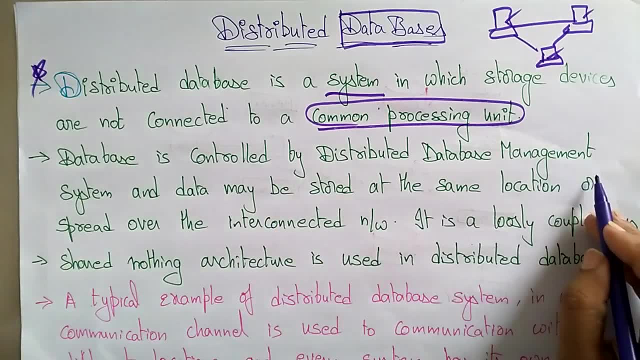 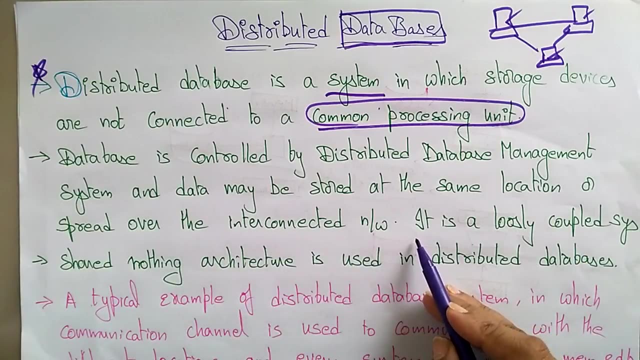 distributed database is a system in which storage devices are not connected to a common processing unit. database is controlled by distributed database management system and data may be stored at same location or spread over the interconnected network. it is loosely coupled system. so what it, they are saying, means here- uh, it is a distributed environment, all the distributed. database managed system and data may be stored at the same location- maybe- okay, maybe- stored at same location or spread over the interconnected network, so that distributed database management system and the data is spreading over to the different systems which are present at different locations through interconnected network. so that's why we call it as a loosely coupled system. 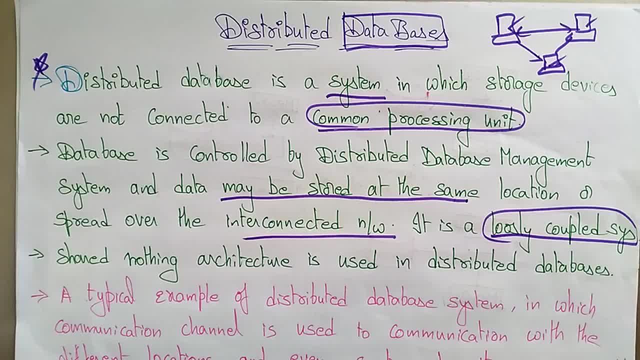 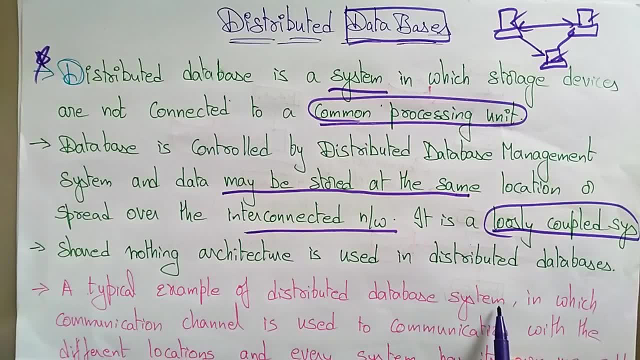 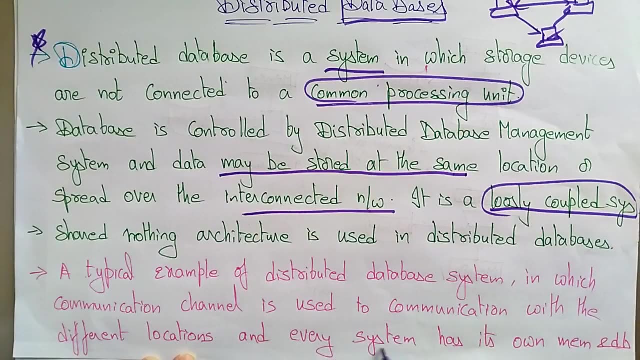 this distributed database is a loosely coupled system so that every system can access the data whenever it required. let's see a typical example of the distributed database system, in which a communication channel is used to communication with the different locations and every system has its own memory and the database. so, for whatever i said now, each system is having their 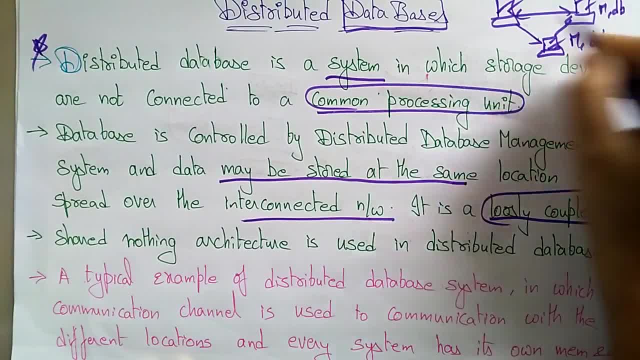 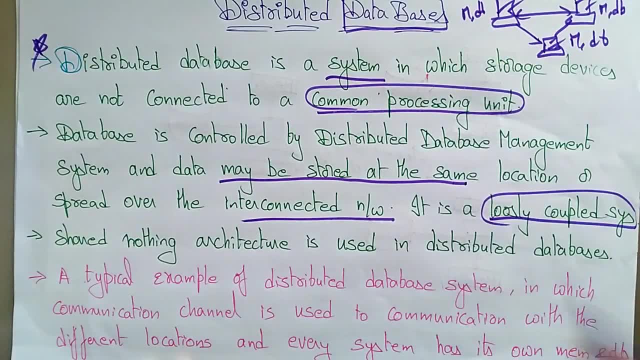 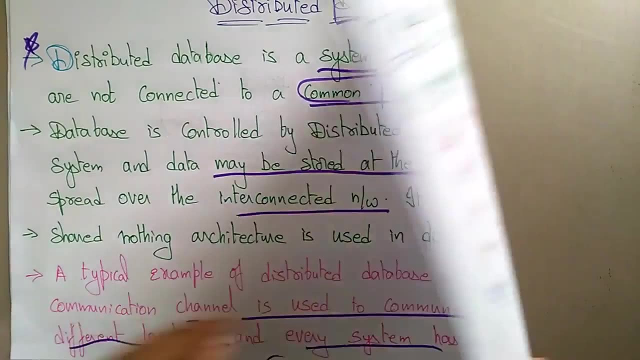 own memory and the database, own memory and the database. so here the main concept is a communication is established, is a communication channel is used to communicate with the different locations, and every system has its own memory and the database. let's see here: this is the diagram of distributed 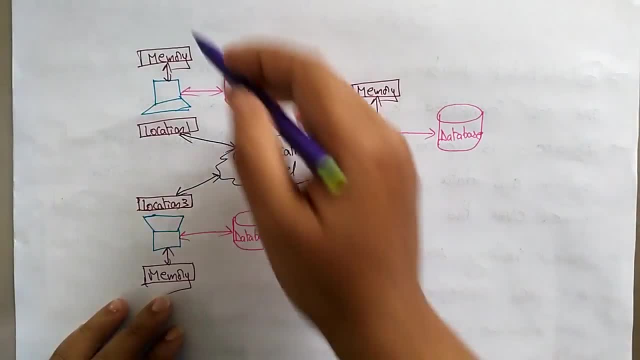 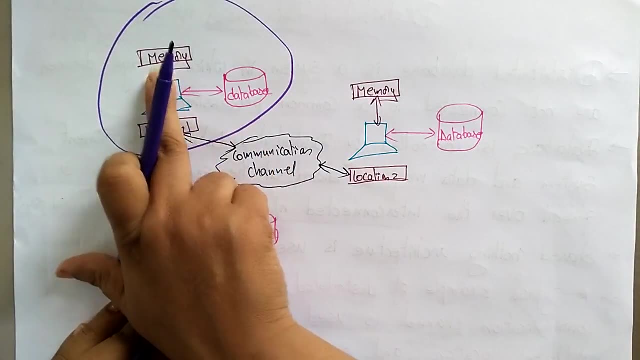 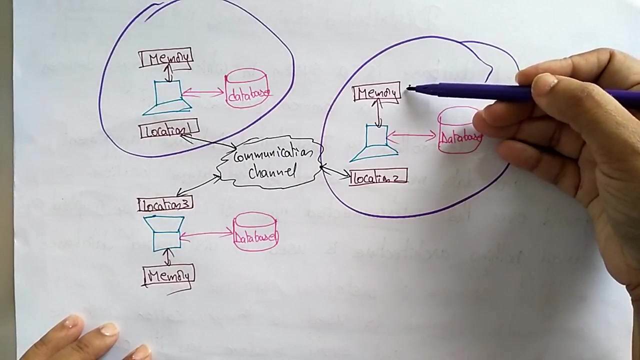 database. so by seeing this picture, what you're understanding here you can see this is one system. this system is present at one location- location one, it's having their own memory and the database- and another system- this system is present at different location, with save outside, with memory and the database, and another. 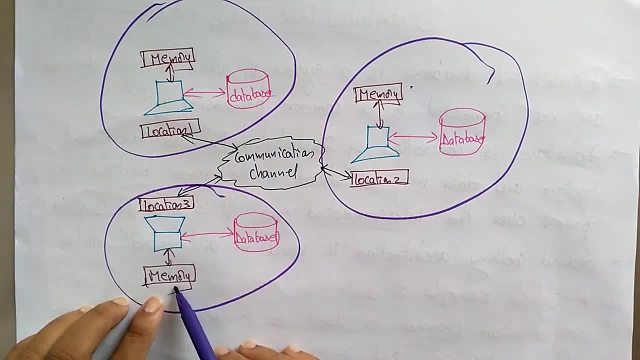 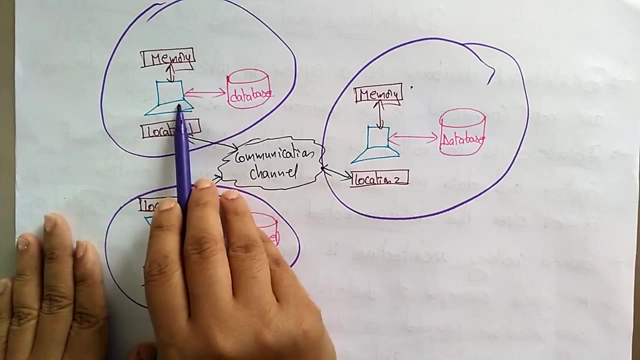 system is stored uh present in different location with the memory and the database. so each system is having their own memory and the database. so this is a distributed environment. here all systems are communicated through this communication channel. so with the help of this communication channel, this database can be accessed here. and this database can be accessed here. 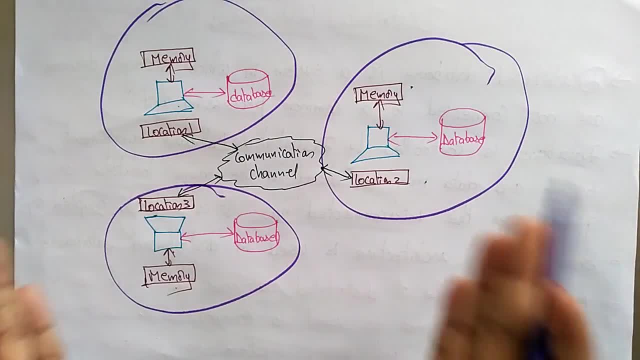 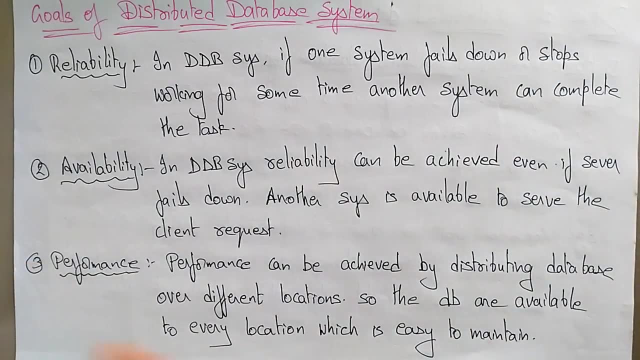 means everything will be communicated. so this is a distributed database environment. let's see the goals of distributed database system. so far, i said what is the distributed database and uh, by showing the diagram, now let's see what are the main goals of distributed database system. why we require this environment? first is reliability.